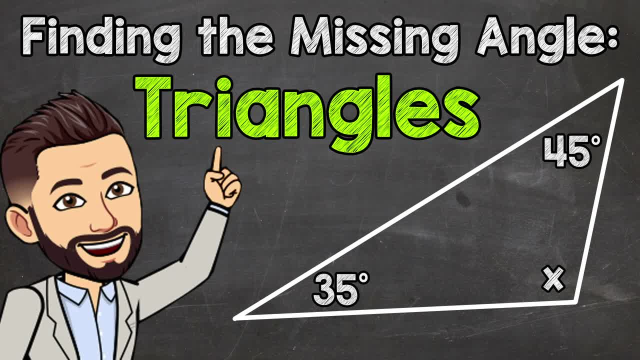 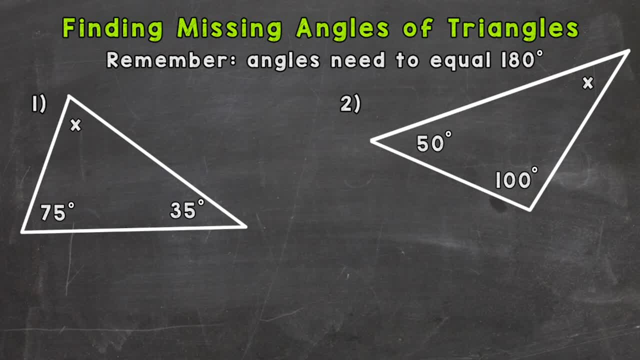 Welcome to Math with Mr J. In this video we're going to be discussing how to find missing angles of triangles And, as you can see, for example, here, there are two triangles on your screen with an x in place of one of the angle measures. So those are our missing angles that we need to. 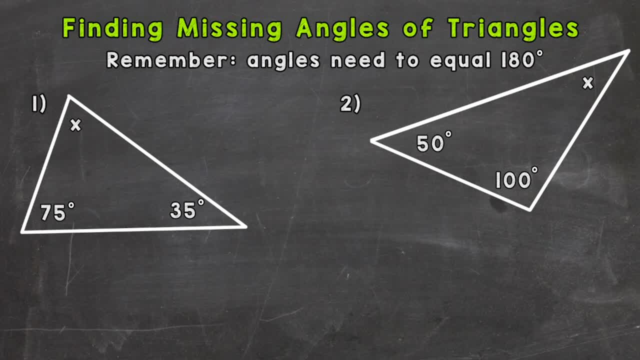 find Now up top is a very important note we need to keep in mind. Remember, angles need to equal 180 degrees, And this 180 degrees is the magic number for every single triangle, no matter what it looks like or how it's classified. When you add the three angles up for a triangle, it's going to 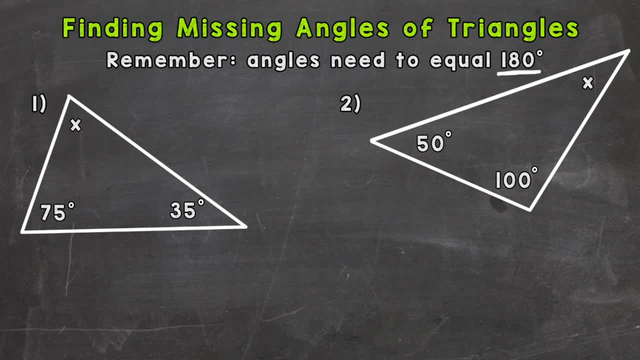 equal 180 degrees. So let's jump right into number one here And see how we find a missing angle. So, like I mentioned earlier, this x is our missing piece within that triangle, our missing angle measure. So the first thing we need to do is take a look at. 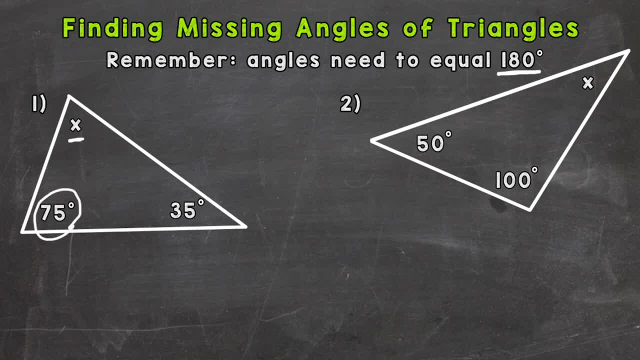 what we are given, And we're given 75 degrees and 35 degrees, So we need to add what we're given together, So 75 plus 35. And that gets us 110 degrees. So we know we have 110 degrees out of the 180 right now. 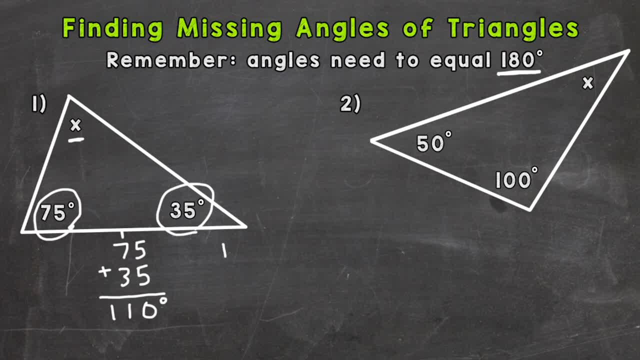 So what we need to do now is take 180 degrees and subtract that 110. And that will give us our missing piece. That x is going to equal 70 degrees. So x equals 70 degrees. Again, we added what we were given: the 75 and 35. That got us to 110 degrees. 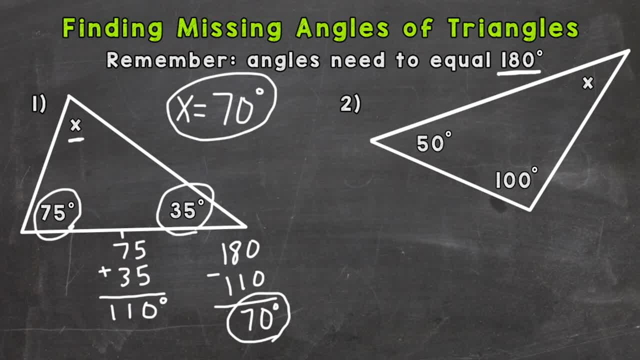 And then we do 180 minus that 110. And it gives us our missing piece. Now, if we do 70 plus the 75 plus the 35, it's going to equal our magic number for triangles: 180 degrees. So let's take a look at number two.